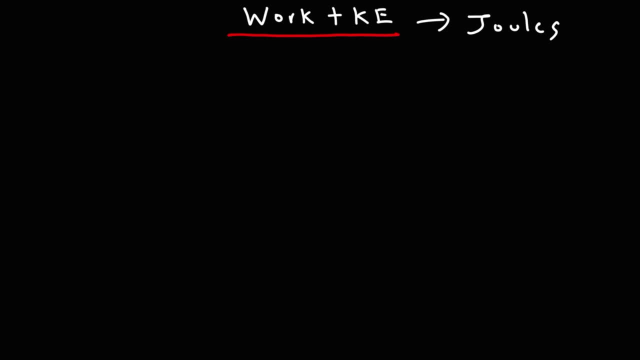 force. the work done by the net force on an object is going to equal the change in the kinetic energy of that object. So in other words, W, the work done by the net force is going to be equal to delta AE. But now let's go ahead and derive this formula: 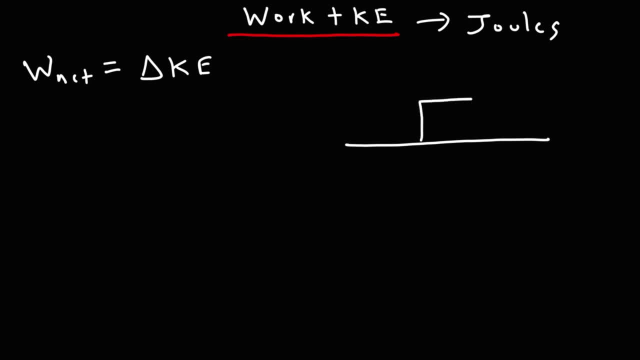 So let's say we have a block resting on a horizontal frictionless surface and we are going to apply coaxial force. So there's only going to be one force in the x direction, so that force will be the same as the. 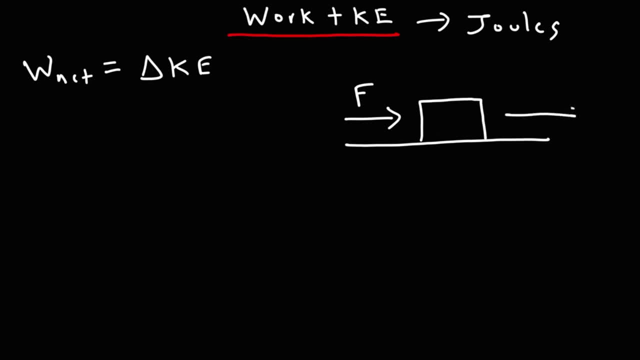 net force And we're going to move this block by some displacement. d. Now the work done by that force is going to be equal to the force times the displacement of the object. Now, because this is the only force acting on the object in the x direction, W is going to represent the network. 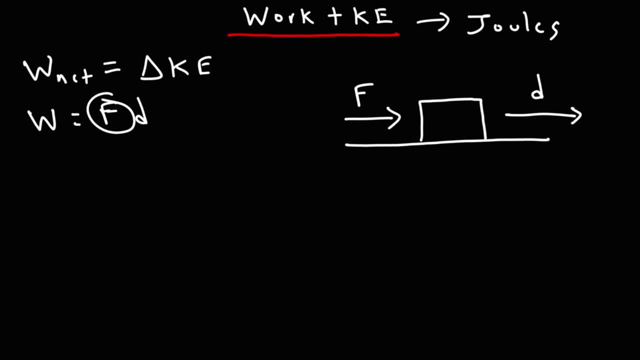 done on the object by that net force. Now, according to Newton's second law, we know that the net force, which in this example is simply F, is equal to mA, So we're going to replace F with mA, So we get this formula. work is mad, mAD. 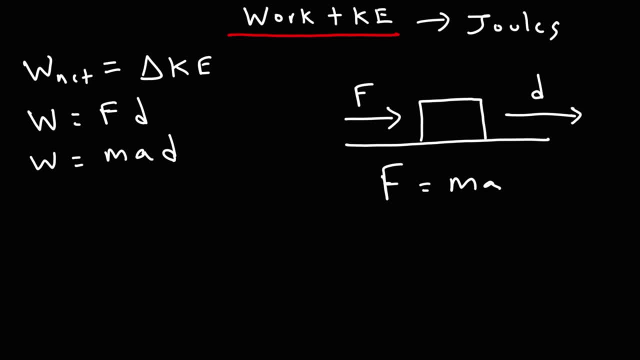 Now let's go ahead and do some math. So here's the net force, which is the force acting on the object, and the displacement, d. Now we're going to replace F with mA, So we get this formula. Work is mad, mAd. 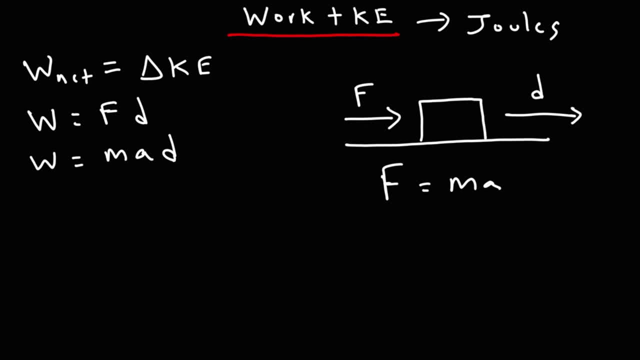 back to our old kinematics equation. We're going to use this one: V final squared is equal to V initial squared plus 2AB. Now we're going to focus on this part: acceleration multiplied by displacement. I'm going to isolate this term in that equation on the right, So I'm going to move. 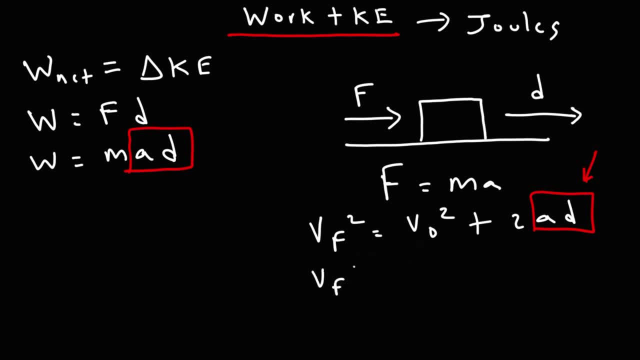 V initial squared to the other side. I'm going to get V final squared minus V initial squared And then to separate the two from AD I'm going to divide both sides by two, So I get that acceleration times. displacement is that it's one half the square differences. 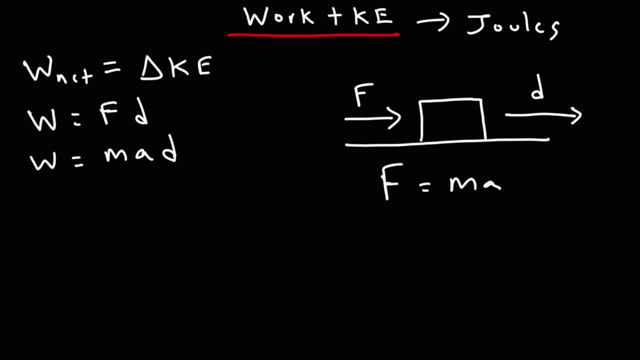 Now let's go back to our old kinematics equation. We're gonna use this: one V final squared is equal to V initial squared plus two AD. Now we're gonna focus on this part: acceleration multiplied by displacement. I'm gonna isolate this term in that equation. on the right: 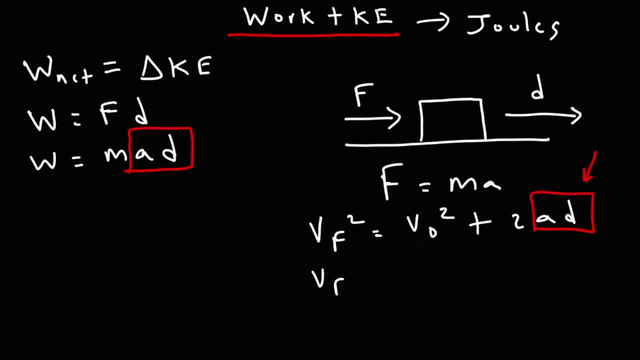 So I'm gonna move V initial squared to the other side. I'm gonna get V final squared minus V initial squared And then to separate the two from AD, I'm gonna divide both sides by two. So I get that acceleration times. displacement is that it's one half the square differences. 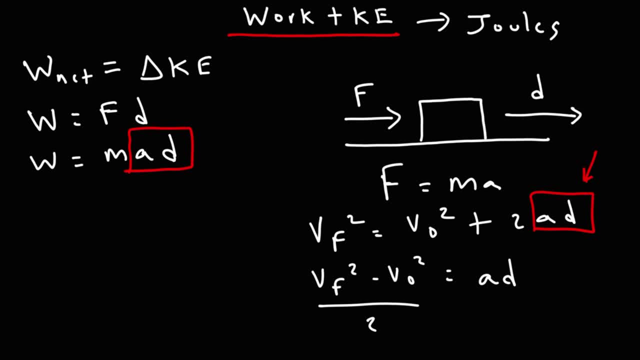 or let me say that again, one half the square difference of final speed and the initial speed. So let's replace AD with what we have here. So now I'm gonna distribute the M and I'm gonna move the two to the front and write it as a half. 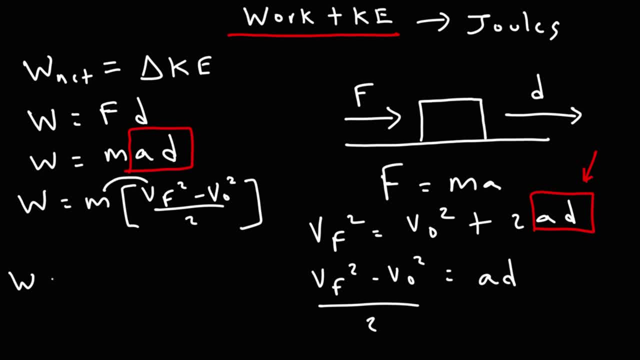 So M times V squared over two, that is one half M V final squared. And then M time negative V initial squared over two is negative: one half M V initial squared. Now we know that kinetic energy is equal to one half M V squared. 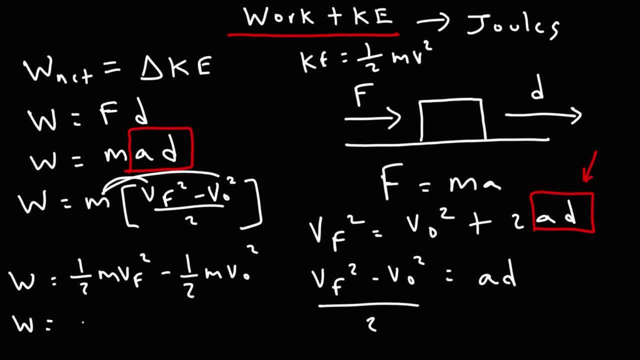 So one half M V final squared, that represents the final kinetic energy, and one half M V initial squared represents the initial, the initial kinetic energy And the final kinetic energy minus the initial kinetic energy. we can replace that with the change in kinetic energy, So that is how we can derive this equation. 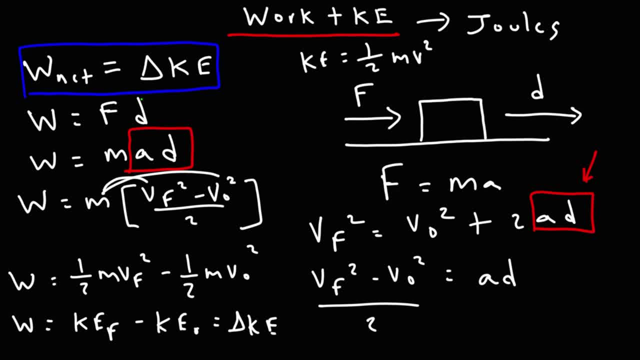 using these two formulas, Work is equal to force times, displacement, and v final squared is equal to v initial squared plus 2ad. So that's how you could derive the work energy theorem. But now let's use an example problem so you could see how they relate to each other. 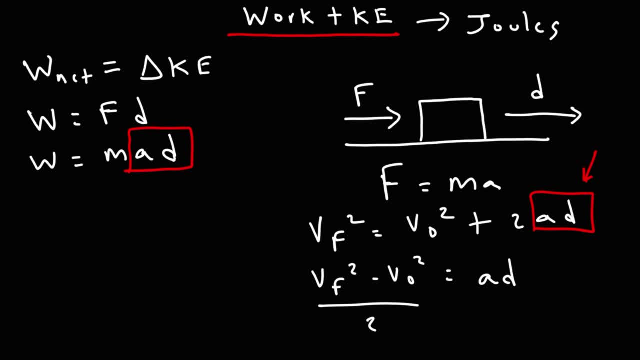 or let me say that again, one half the square difference of final speed and the initial speed. So let's replace A AD with what we have here. So now I'm going to distribute the M and I'm going to move the two to the front. 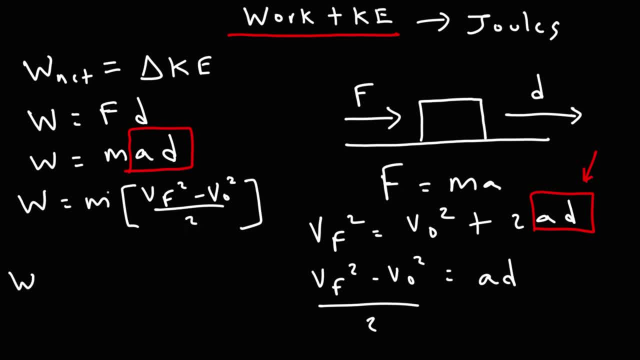 and write it as a half. So M times V squared over two, that is one half M V final squared. And then M times negative V initial squared over two is negative: one half M V initial squared. Now we know that kinetic energy is equal to one half M V squared. 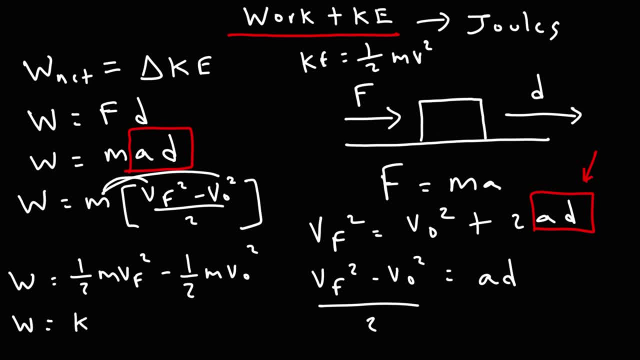 So one half M V final squared, that represents the final kinetic energy, And one half M V initial squared represents the initial kinetic energy And the final kinetic energy minus the initial kinetic energy. we can replace that with the change in kinetic energy, So that is how we can derive this equation. 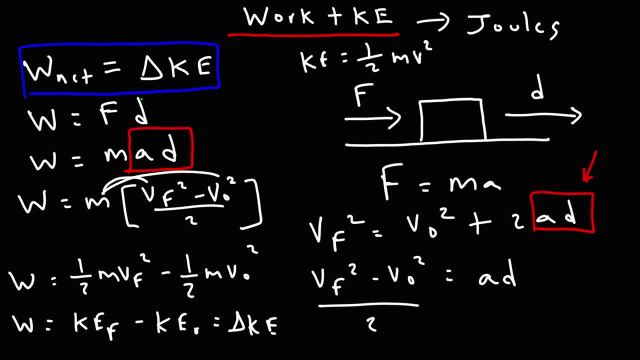 using these two formulas, Work is equal to force times, displacement, And V final squared is equal to V initial squared plus two AD. So that's how you could derive the work energy theorem. But now let's use an example problem So you could see how they relate. 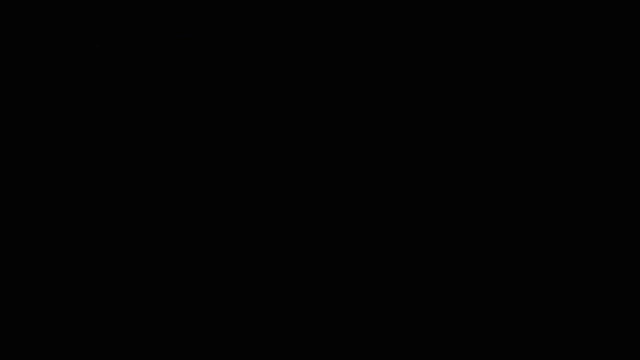 to each other. So let's say we have a horizontal frictionless floor and we have a 10-kilogram block and we're going to apply a force of 90 Newtons on this block And let's say, initially this block is moving to the right at a speed of 4 meters per second. 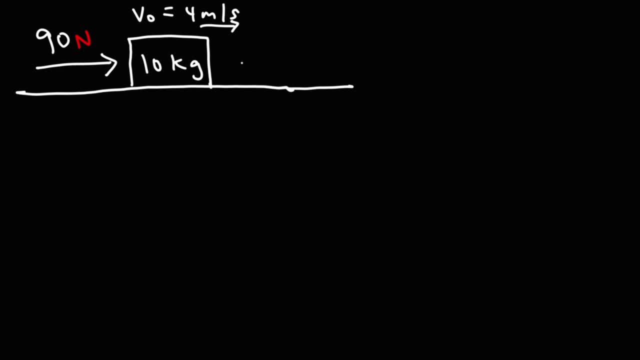 Now we're going to apply this 90-Newton force for a displacement of 20 meters. Go ahead and calculate the work done by this force using. do it two ways. Now, the first method is pretty straightforward: The work done by this force on the block is simply force times displacement. 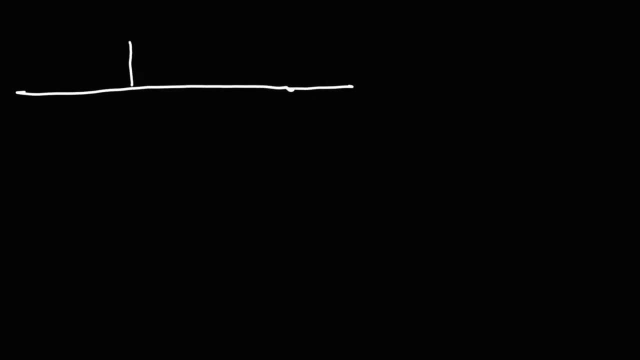 So let's say we have a horizontal frictionless floor and we have a 10-kilogram block and we're going to apply a force of 90 newtons on this block. And let's say initially this block is much more than 90 newtons. 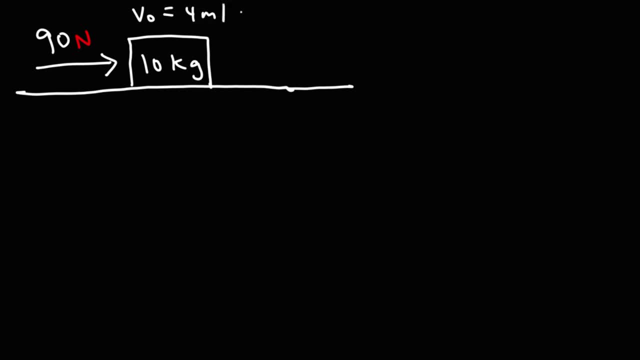 And we're going to apply a force of 90 newtons on this block- And let's say initially this block is much more than 90 newtons- moving to the right at a speed of four meters per second. Now we're going to apply this 90. 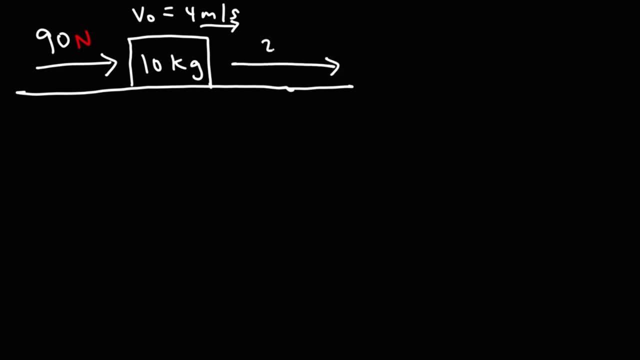 Newton force for a displacement of 20 meters. Go ahead and calculate the work done by this force using. do it two ways. Now, the first method is pretty straightforward. The work done by this force on the block is simply force times displacement. So it's going to be 90 Newtons. 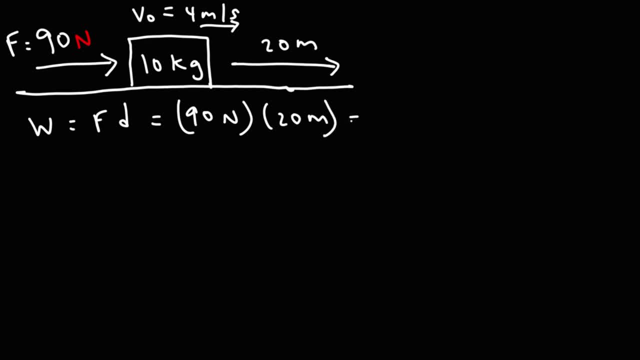 times 20 meters, 9 times 2 is 18.. If we carry over the two zeros, we get 1800 Newton meters, which is 1800 joules. Now let's calculate the work by using the change in kinetic energy formula. 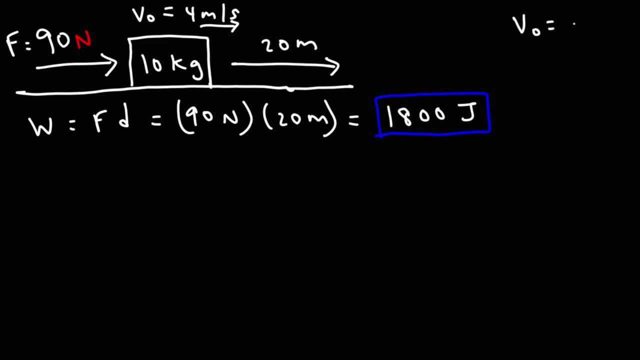 So we know the initial speed is 4 meters per second. We need to determine the final speed Now. using F is equal to ma. we can calculate the acceleration. So the acceleration is going to be force over mass. So we have 90 Newtons of force acting on a 10 kilogram. 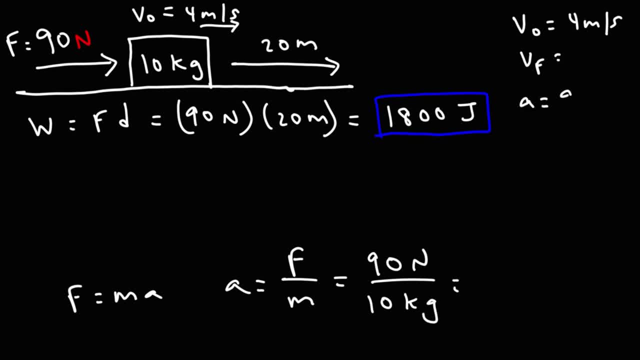 object And that will give us an acceleration of 9 meters per second squared. Now, using this formula, V final squared is equal to V initial squared plus 2ad. We can calculate the final speed. So V initial is 4.. Acceleration is 9.. The displacement is 20.. 4 squared is 16.. 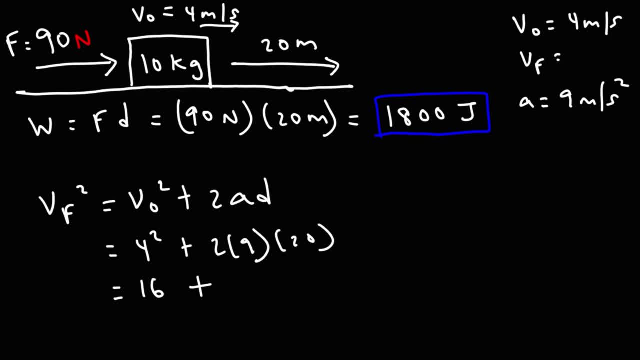 20 times 9 is Well, two times 9 is 18.. So 20 times 9 is 180. times 2, that's 360.. So we get V. final squared is 376.. So now let's take the square root of that value. That's going to give us 19.3.. 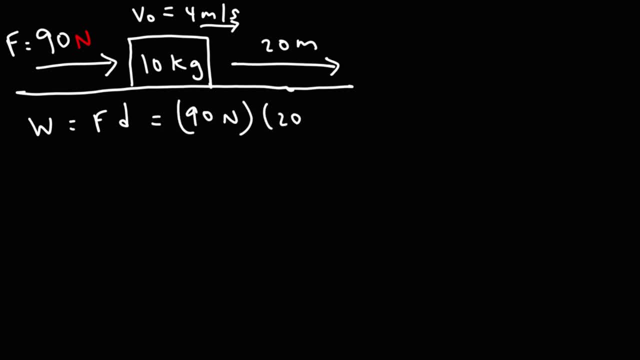 So it's going to be 90 Newtons. 90 Newtons times 20 meters, Nine times two is 18.. If we carry over the two zeros, we get 1,800 Newton meters, which is 1,800 joules. 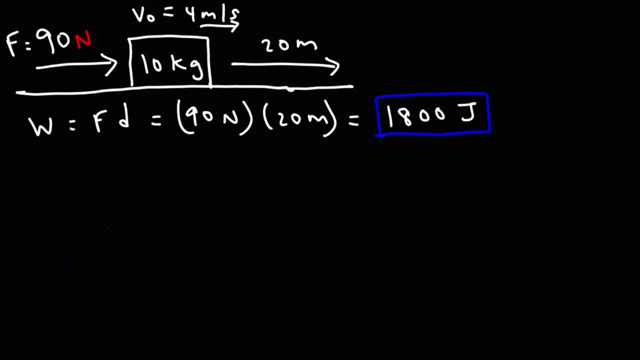 Now let's calculate the work by using the change in kinetic energy formula. So we know the initial speed is 4 meters per second. We need to determine the final speed Now. using F is equal to MA, we can calculate the acceleration. 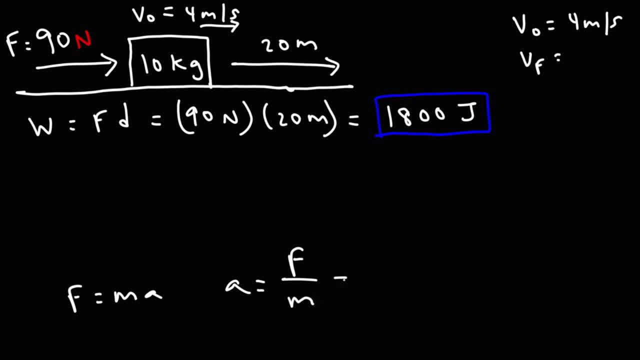 So the acceleration is going to be force over mass. So we have 90 Newtons of force acting on a 10-kilogram object and that will give us an acceleration of 9 meters per second squared. Now, using this formula, V final squared is equal to V initial squared plus 4 meters per 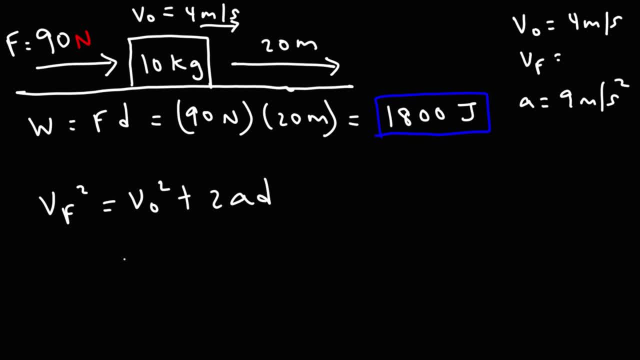 second squared plus 2 AD, We can calculate the final speed. So V initial is 4.. Acceleration is 9.. The displacement is 20.. Four squared is 16.. 20 times 9 is well, 2 times 9 is 18.. 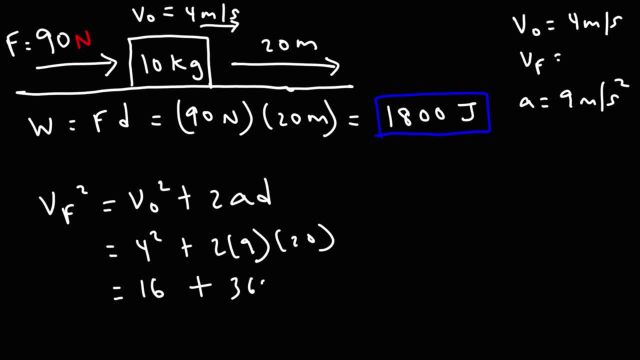 So 20 times 9 is 180.. Times 2,, that's 360.. So we get V. final squared is 376.. So now let's take this formula. Okay, Let's take the square root of that value. That's going to give us 19.3907 meters per second squared. 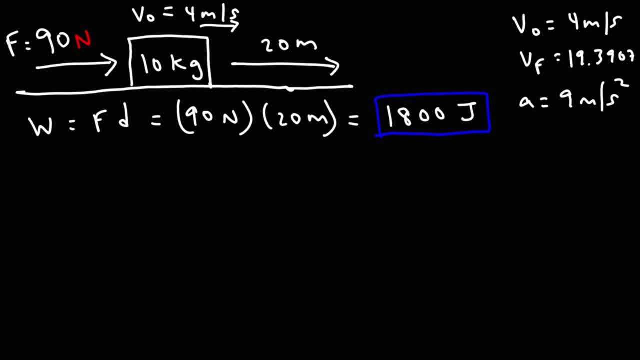 I mean just meters per second. So now we could use this formula to calculate the work. It's going to be the final kinetic energy minus the initial kinetic energy, So that's going to be 1 half MV final squared minus 1 half MV initial squared. 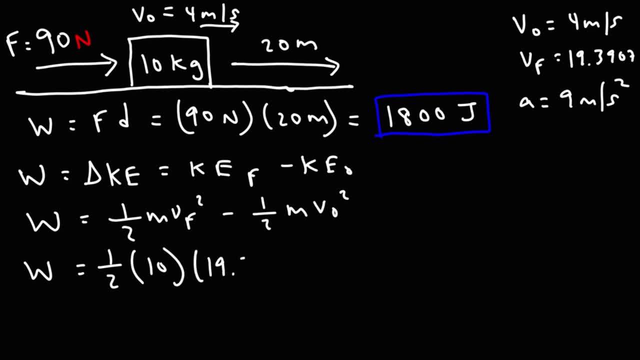 So the mass is 10.. V final is 19.3907 meters per second And the initial speed is 4.. So that's going to be 1 half MV final squared minus 1 half MV initial squared, So the mass is 10.. 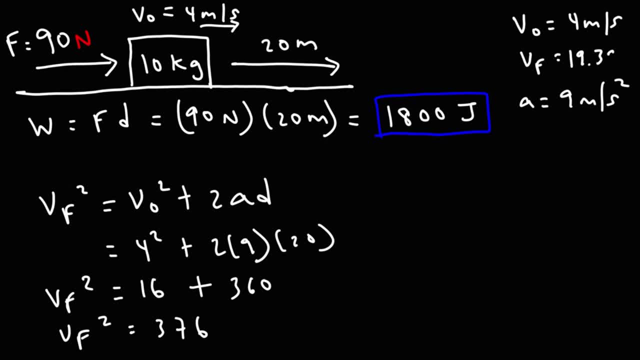 That's going to give us 19.3. 19.3. 19.3. 19.3. 19.3. 19.3.. three nine zero seven meters per second score. i mean just meters per second. so now we could use this formula to calculate the work. 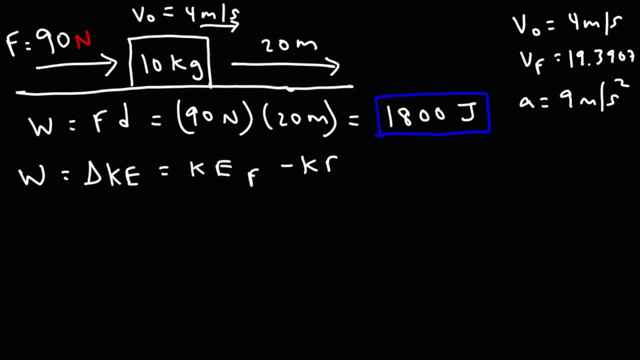 it's going to be the final kinetic energy minus the initial kinetic energy, so that's going to be one half mv final squared minus one half mv initial squared. so the mass is 10 v final is 19.3907 meters per second and the initial speed is 4.. 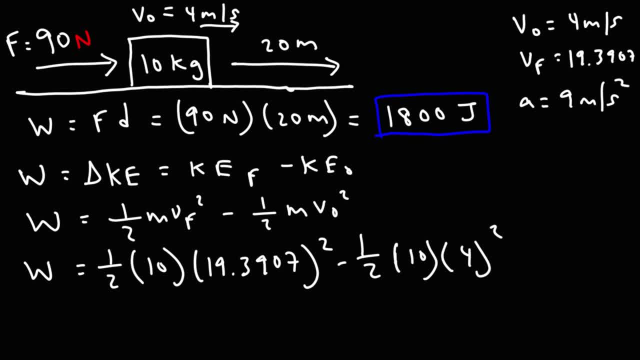 so 19.3907. we know that once we square it, we're going to get 376 times half of 10, which is 5.. so that's going to give us 3 entender. now, four squared is 16 times 10, that's 160. half of 160 is 80.. 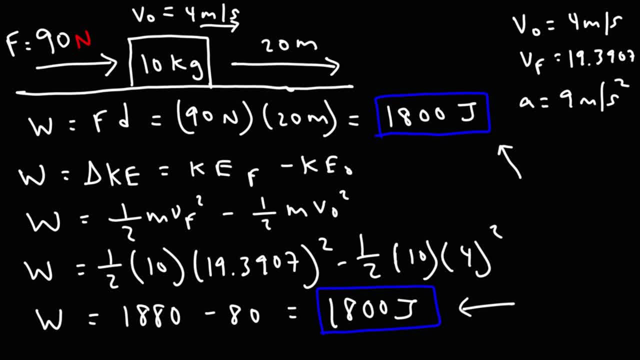 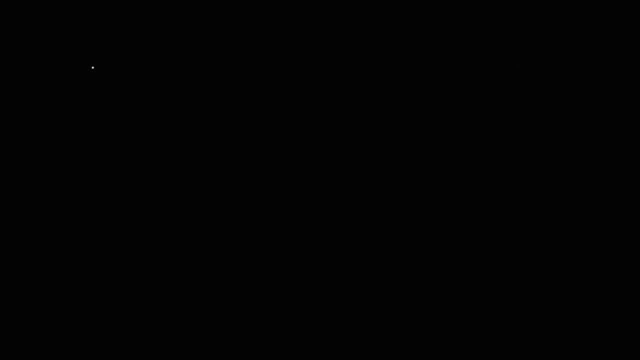 so we get the same answer. but that's how you can calculate the work done by a force answer: by calculating the change in kinetic energy. now let's work on a similar problem. so this time we're going to have a five kilogram mass on a horizontal frictionless floor and we're going to apply a force of 40 Newtons. 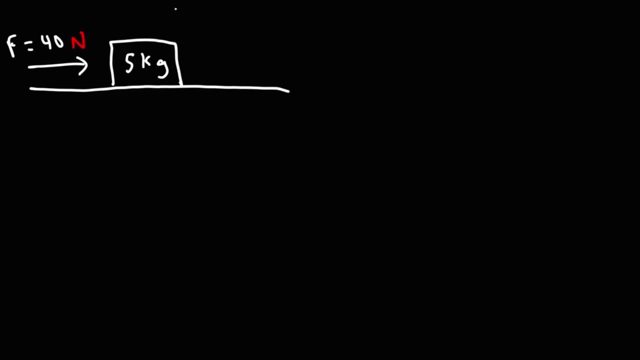 now, initially, this block will be at rest, so it's going to accelerate from rest and we're going to apply this force for a time period of eight seconds. what is the work done by this force? so in this problem, we're not given the displacement of the object, or that the object travels through while the force. 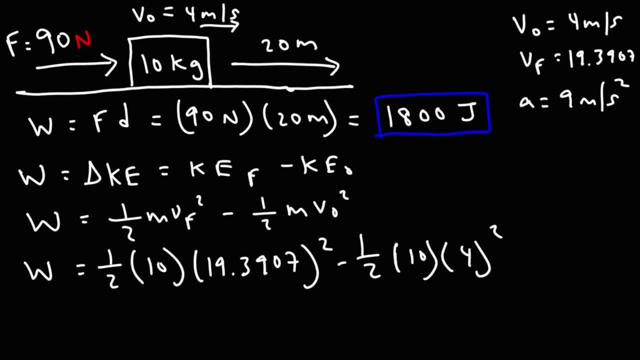 The final is 19.3907 meters per second, So 19.3907.. We know that once we square it we're going to get 376 times half of 10, which is 5.. So that's going to give us 1880.. 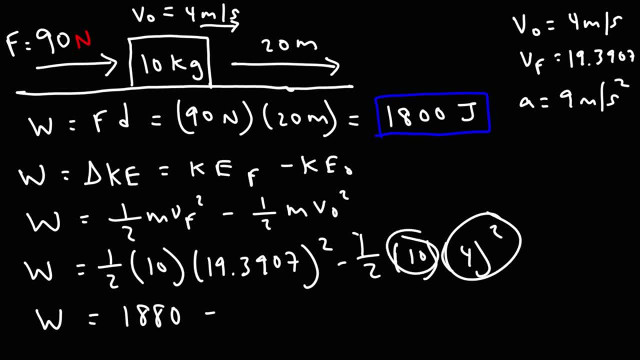 Now, 4 squared is 16 times 10. That's 160.. Half of 160 is 80.. 1880 minus 80 is 1800.. So, as we can see, we get the same answer. But that's how you can calculate the work done by a force. 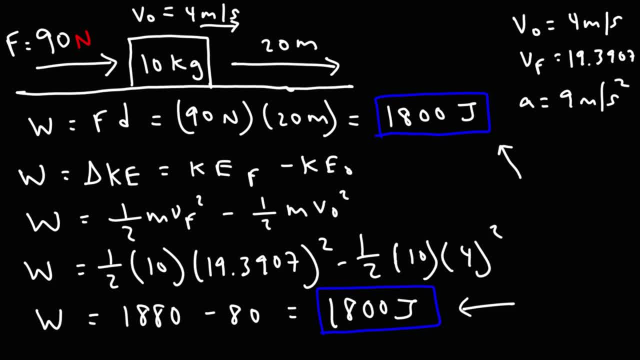 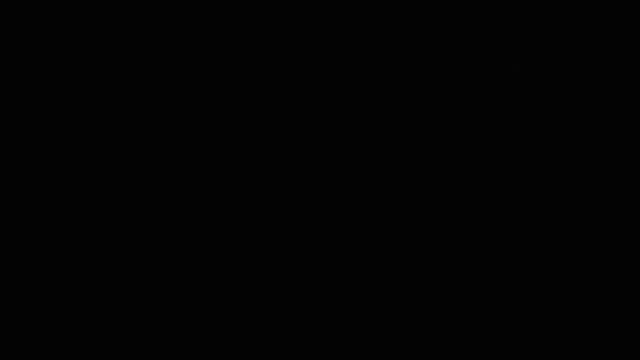 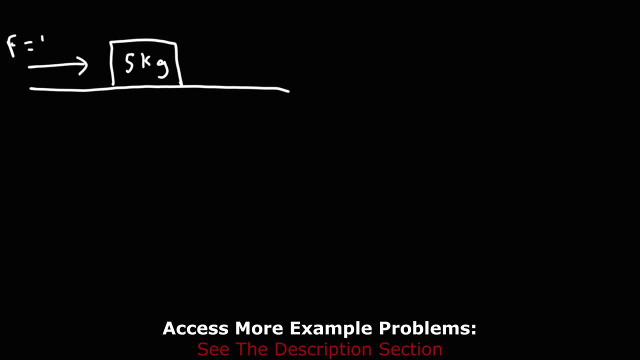 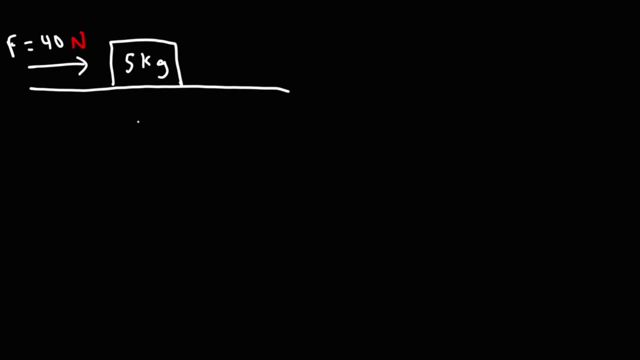 Now, initially, this block will be at rest, So it's going to accelerate from rest And we're going to apply this force for a time period of 8 seconds. What is the work done by this force? So in this problem, we're not given the displacement of the object. 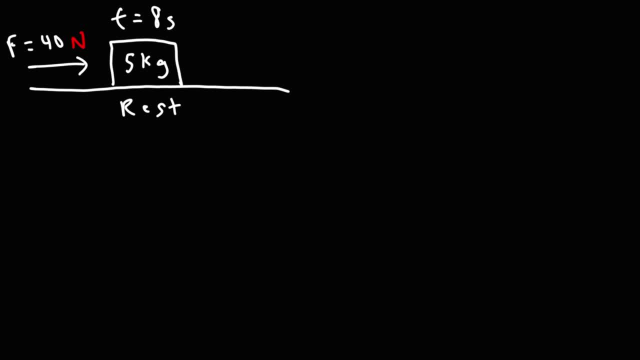 or that the object travels through while the force is acting upon it. So feel free to pause the video and calculate the work done using both methods. The first thing I would do is calculate the acceleration. So we have a force of 40 Newtons acting on a 5 kilogram object. 40 divided by 5 is 8.. So we get an acceleration of 8 meters. 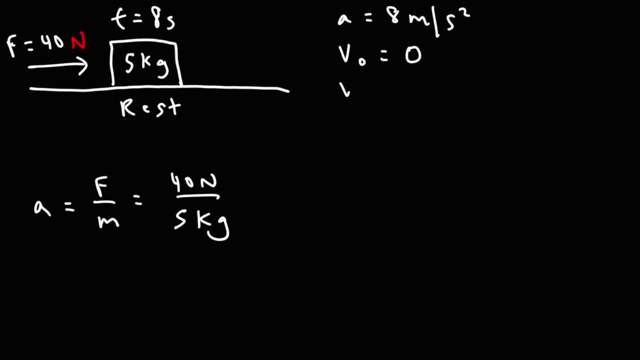 per second squared. We know the initial velocity is 0, but we can calculate the final velocity Using this formula: V final is equal to V initial plus A t. V initial is 0.. We've got an acceleration of 8 meters per second squared, which means that every second 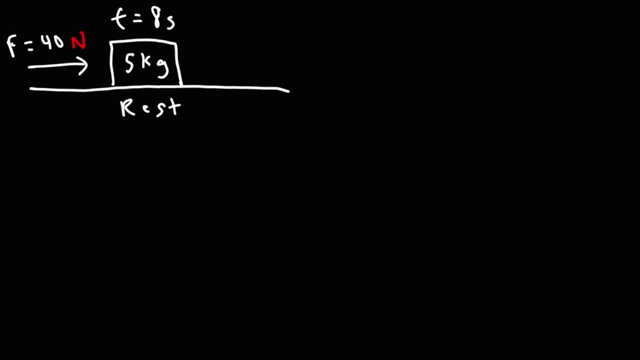 is acting upon it, so feel free to pause the video and calculate the work done using both methods. the first thing I would do is calculate the acceleration. so we have a force of 40 Newtons acting on a 5 kilogram object. 40 divided by 5 is 8, so 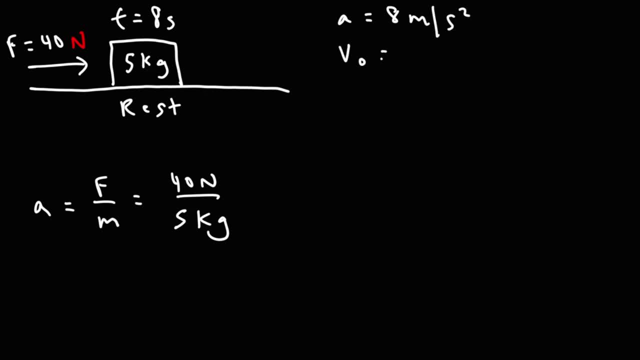 we get an acceleration of 8 meters per second squared. we know the initial velocity is zero, but we can calculate the final velocity using this formula: the final is equal to the initial plus 80. the initial is 0. we've got an acceleration of 8 meters per. 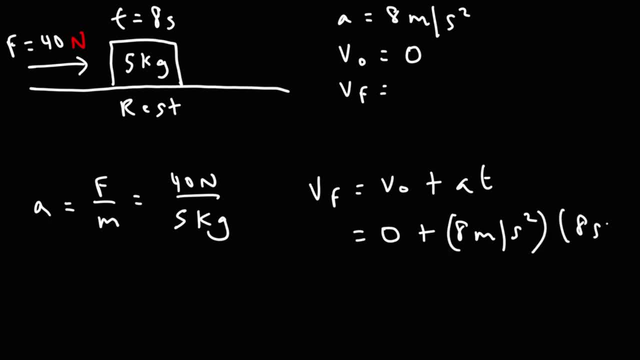 second squared, which means that every second the velocity will increase by 8. so 8 times 8, 64. so that's going to be the final velocity. now calculate the displacement, since we know the initial and the final velocity, as well as the time. So the initial velocity is 0,, the final velocity is 64, the time: 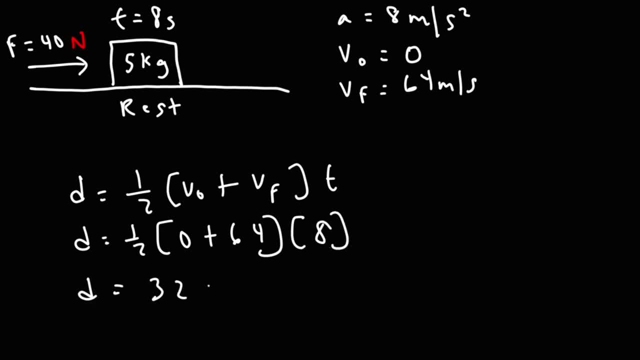 is 8.. Half of 64 is 32, so this is going to be 32 times 8.. 32 times 8 is 256.. So that's going to be the displacement. That's how far this block is going to travel in 8 seconds with a 40 Newton force acting upon it. So now let's calculate. 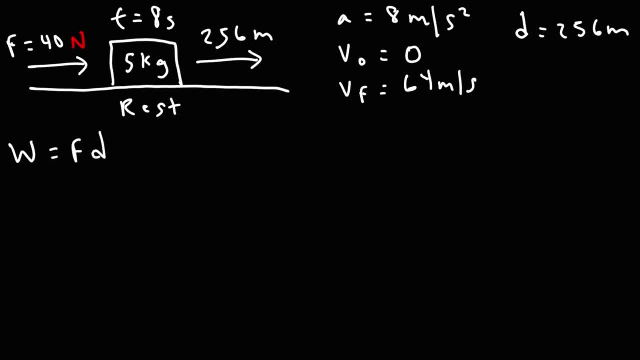 the work. So the work done by the force is going to be force times displacement, which is 40 Newtons. This is going to be force times 256 meters. So that's going to give us 10,240 Joules. Now let's use the work Energy theorem to calculate the work done by the 40N force. So this is: 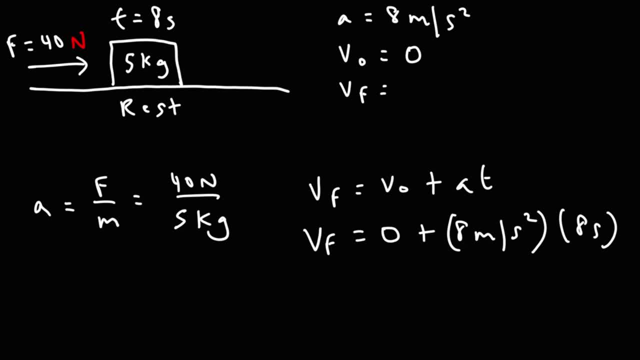 is equal to V initial plus A t. V initial is 0.. We've got an acceleration of 8 meters per second. squared, The velocity will increase by 8.. So 8 times 8 is 64.. So that's going to be the final. 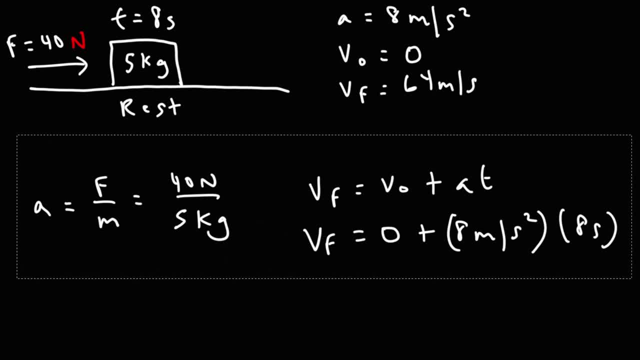 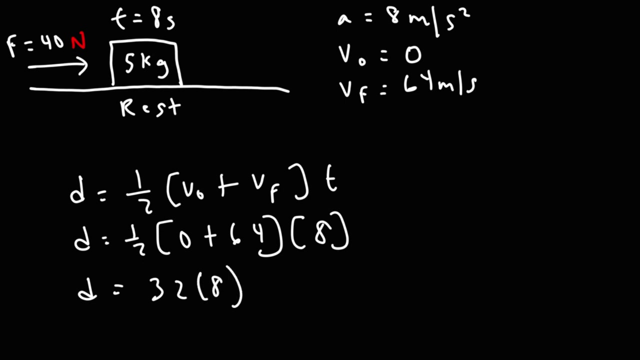 velocity. Now we can calculate the displacement, since we know the initial and the final velocity, as well as the time. So the initial velocity is 0, the final velocity is 64. The time is 8. Half of 64 is 32.. So this is going to be 32 times 8.. 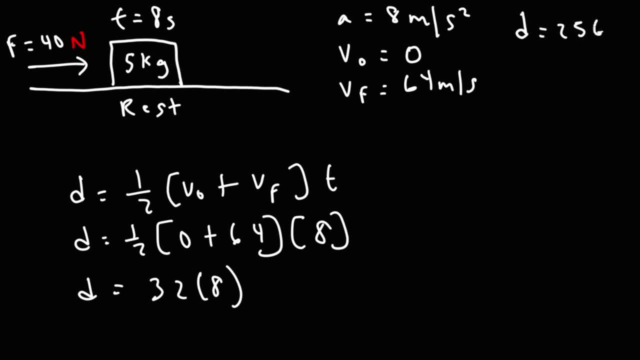 32 times 8 is 256.. So that's going to be the displacement. That's how far this block is going to travel in 8 seconds with a 40-newton force wrapped in upon it. So now let's calculate the work. 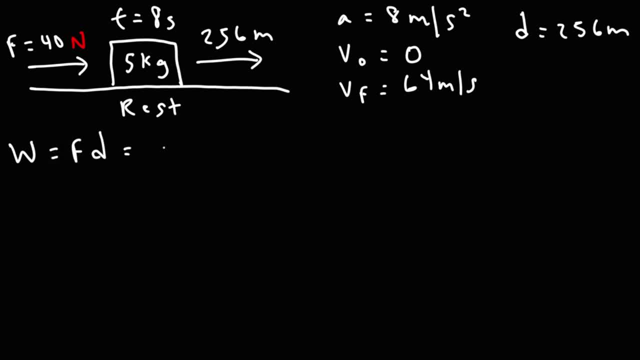 So the work done by the force is going to be force times displacement, which is 40 newtons times 256 meters. So that's going to give us 10,240 joules. Now let's use the work energy theorem to calculate the work done by the 40-newton force. 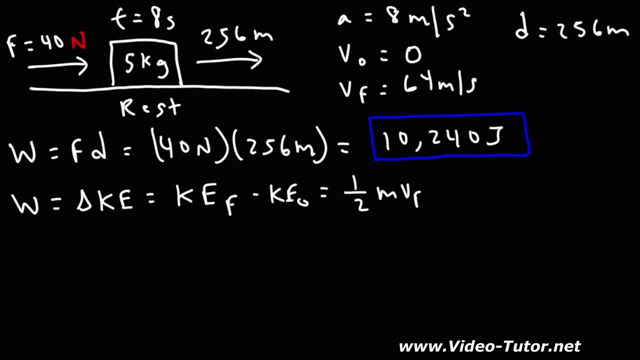 So this is going to be 1 half mv final squared minus 1 half mv initial squared, So the mass is 5, the final velocity is 64.. The initial velocity is 0, so this disappears. The work is simply equal to the final kinetic energy in this problem. 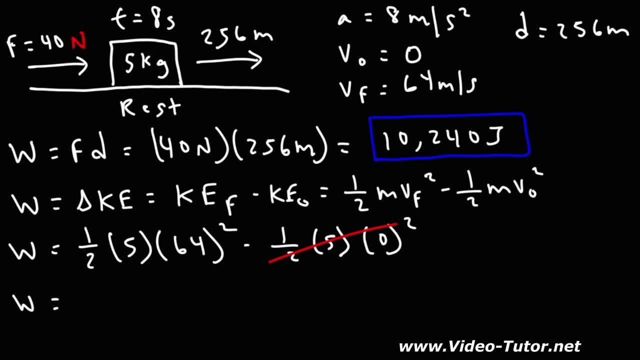 So 0.5 times 5 times 64, squared, will give us the same answer of 10,240 joules. So those are two simple ways in which you can calculate the net work done by a force or the work done by a net force. 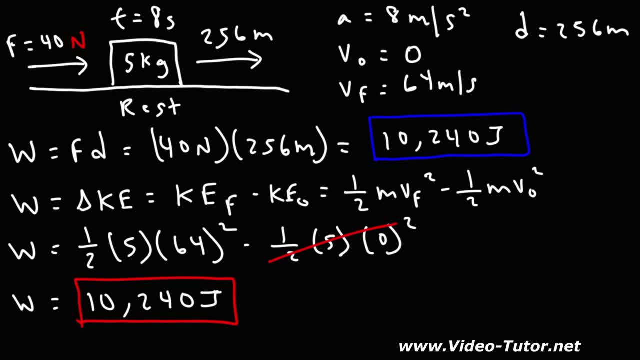 You could use the force times displacement formula or you can calculate the work done by calculating the change in the object's kinetic energy.